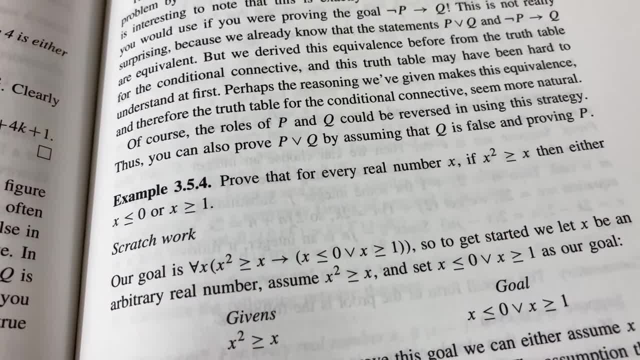 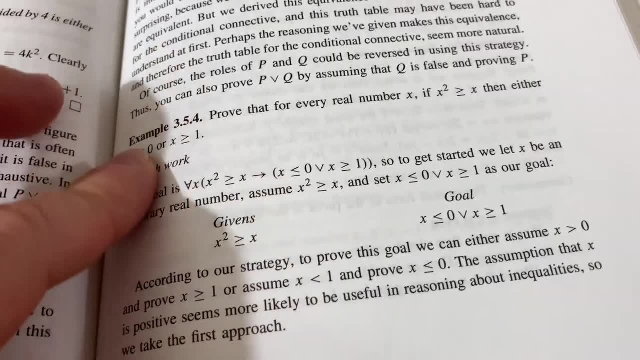 It says: prove that for every real number, x. if x, squared is greater than or equal to x, then either x is less than or equal to zero, or x is greater than or equal to one. And what I like about this book is that he breaks down the scratch work, and that's exactly what I 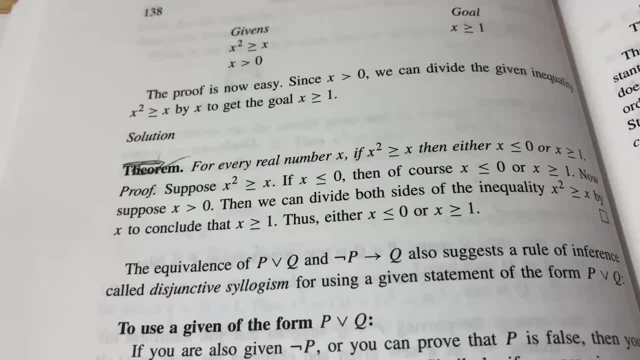 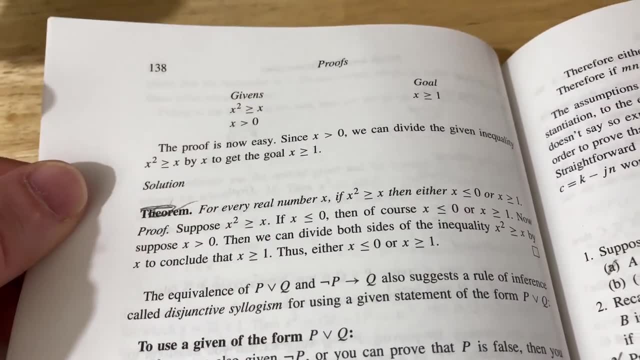 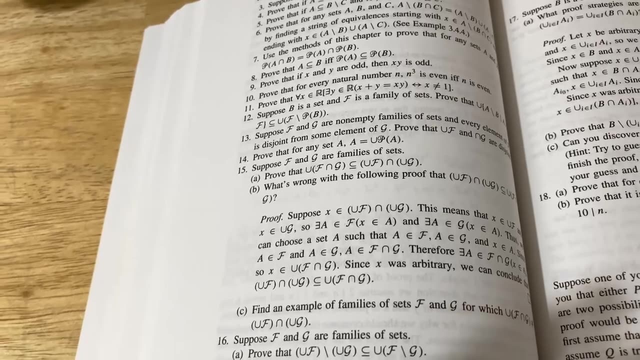 call it when I'm working on proofs, which I think is super cool. Then here he states it as a theorem and goes through the proof, So he actually shows you how to figure out the proofs, and he does it in incredible detail. This book also has tons of exercises, which I think is really good if you're looking for extra. 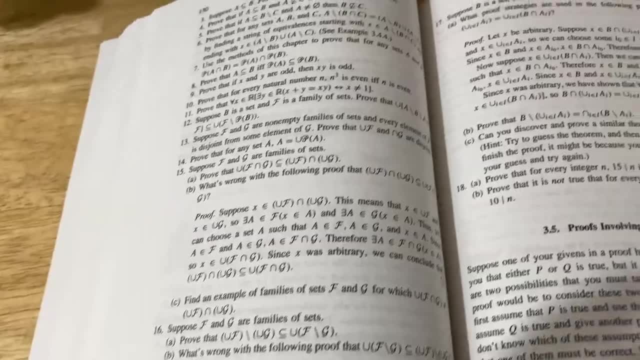 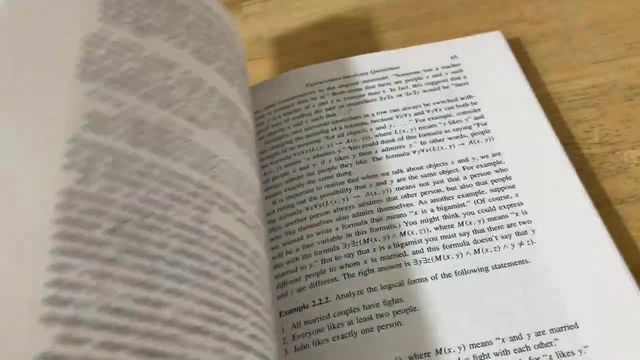 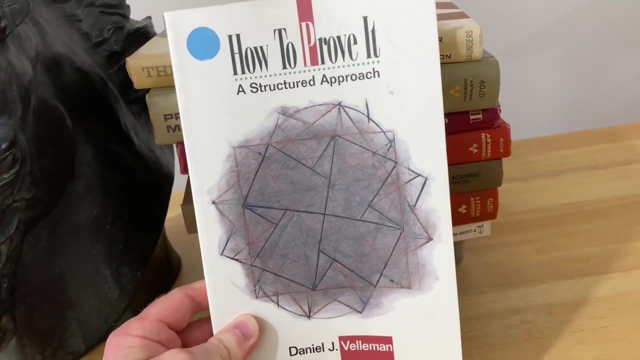 practice problems. One of the downsides, though, is that it does not contain solutions to any of the exercises. Just gotta give it a whiff. Yeah, my copy smells fairly new. Okay, let's do a little bit of logic, and I'm going to explain why those statements I mentioned at the beginning of the 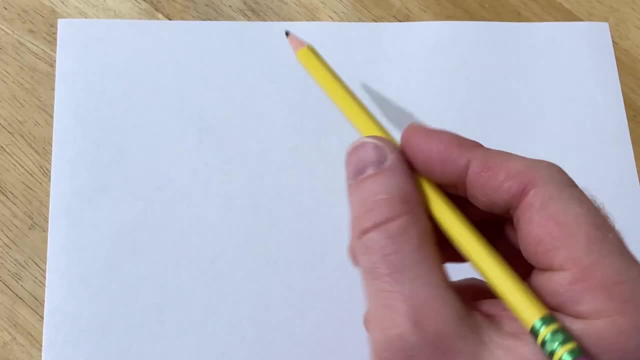 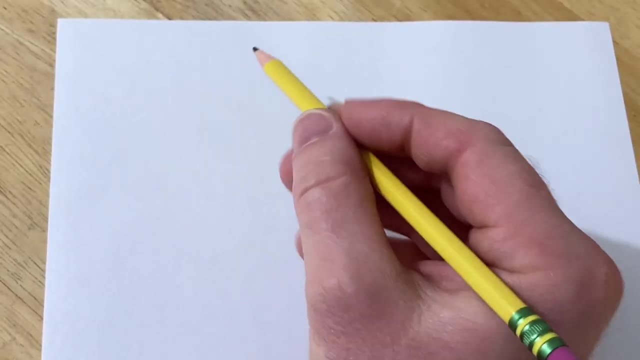 video are actually true. In order to understand the stuff I was talking about during the beginning of this video, you have to know a little bit of mathematical logic. So let me just show you so that you can understand why statements like all unicorns can do math or all unicorns are purple. 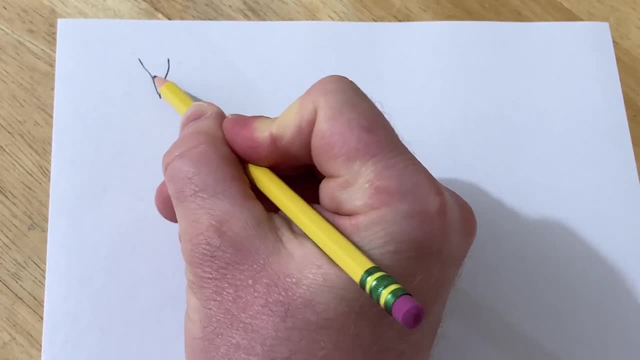 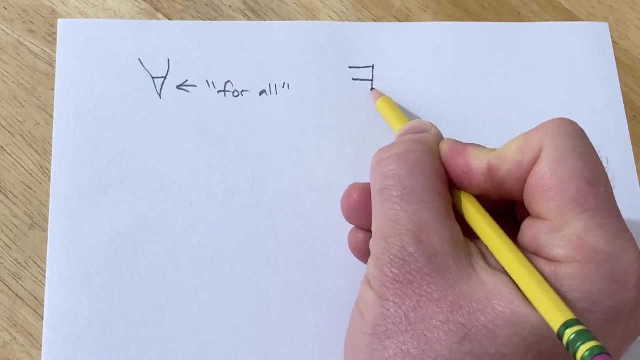 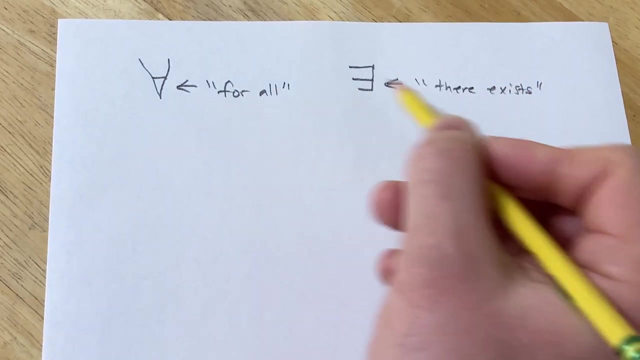 are actually true mathematically. So this upside down A, this symbol means for all, And this backwards E, this symbol means there exists. These are examples of things we call quantifiers in mathematics. All right, I'm going to let A be. 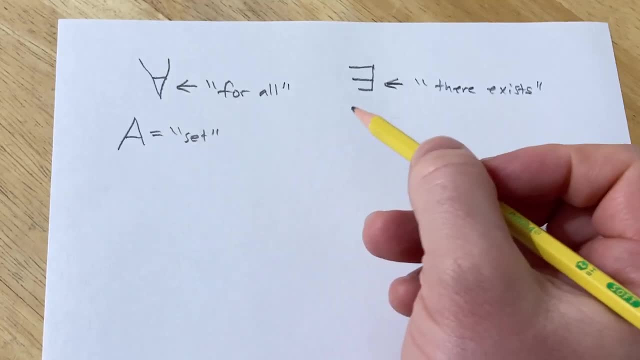 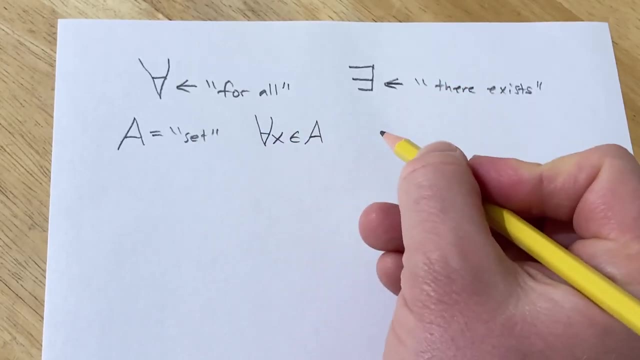 equal to a set. A set is just a collection of objects. So if I write for all X in A, that's exactly how you read it And this symbol here is read is in belongs to. I just read it for all X. 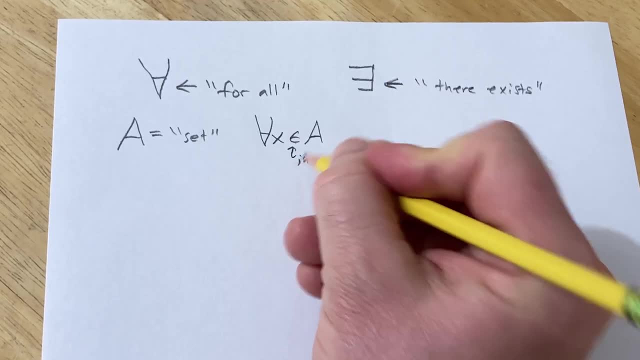 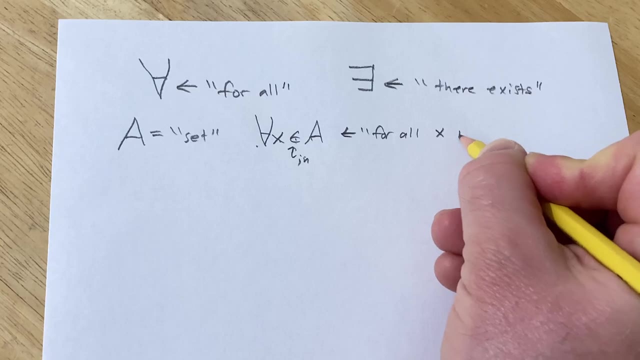 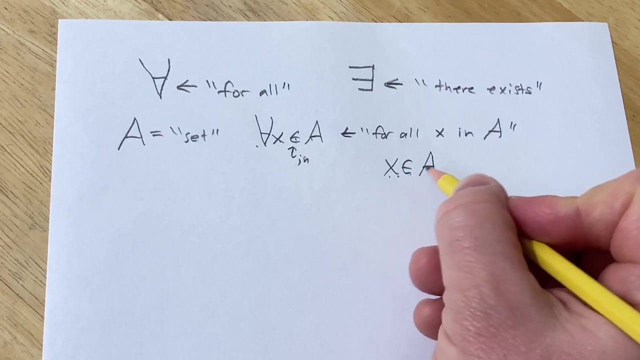 in A. So in in, in, So for all X in A. So if someone just says X in A, you can say X is in A. You can say X is an element of A, X belongs to A, X is a member of A. So there's a bunch of different ways to say it, But typically when you 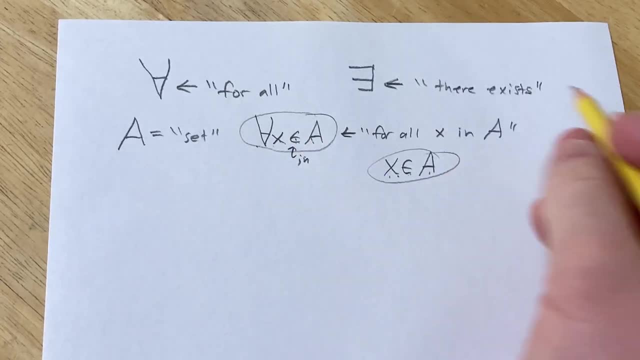 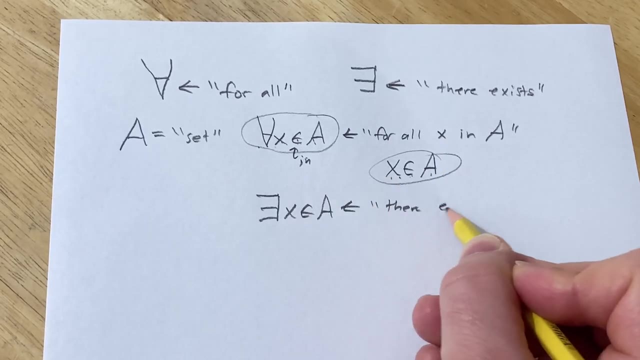 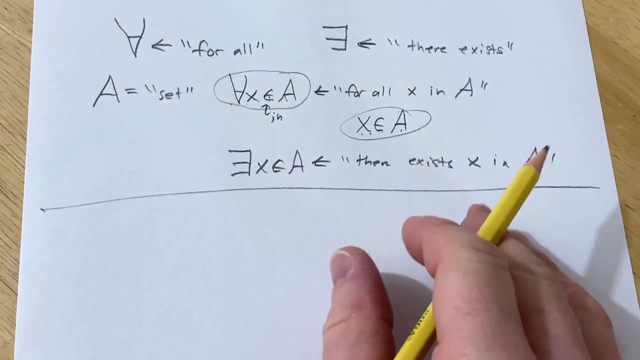 look at it. you just say: for all X in A, And then, if someone does this, this means there exists. You can say: for all X in A. Okay, So there's a bunch more logic. You actually need to like fully understand this. So I'm just 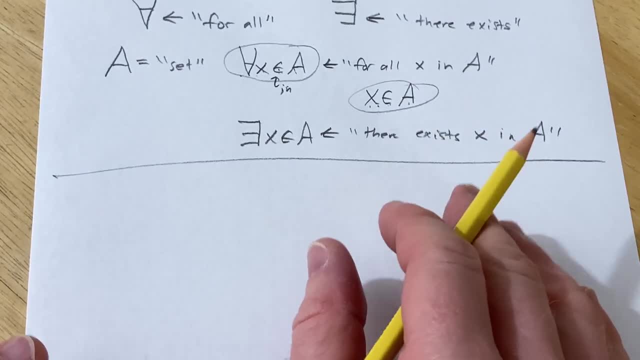 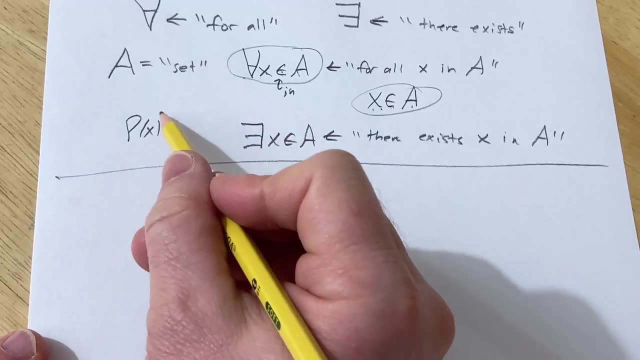 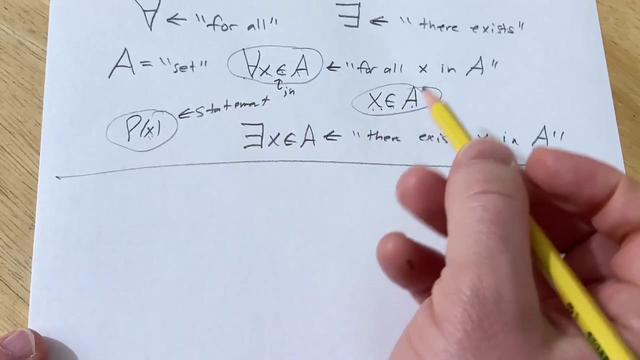 gonna jump into it now and do my best to explain, And hopefully it makes sense. By the way, if someone writes P of X, this is a statement. We don't know if it's true, We don't know if it's false. This is a statement that depends on X. So this is going to be a statement, All right. So 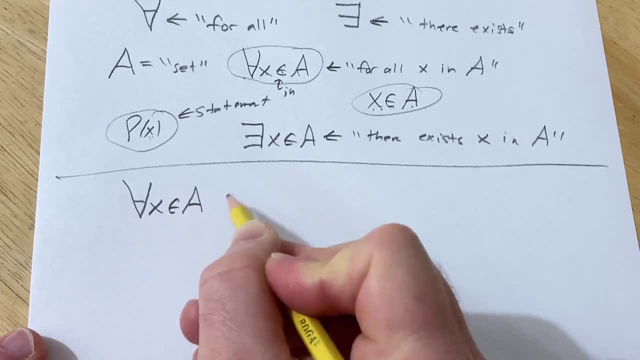 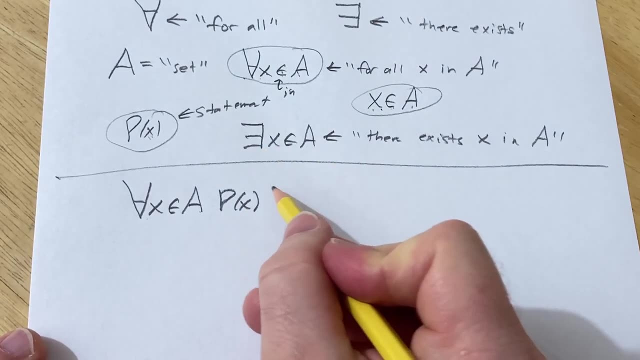 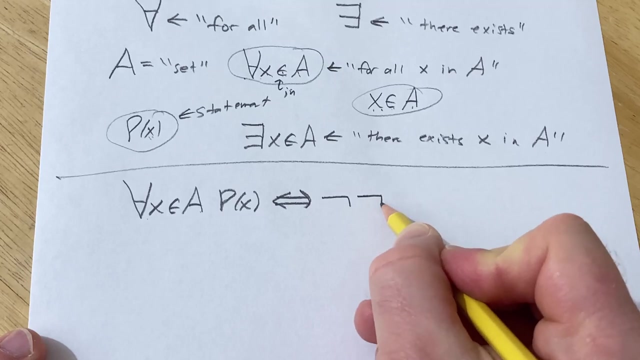 for all x and a p of x. we're saying that for all x and a. we're investigating the statement p of x. This is the same as saying so I'm going to write a little symbol here, the opposite of, the opposite of for all x and a p of x. So this is a negation symbol. 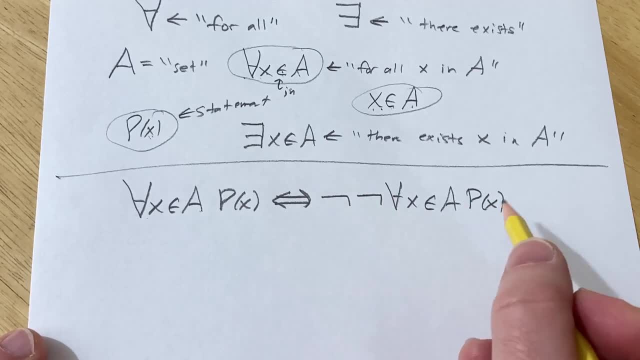 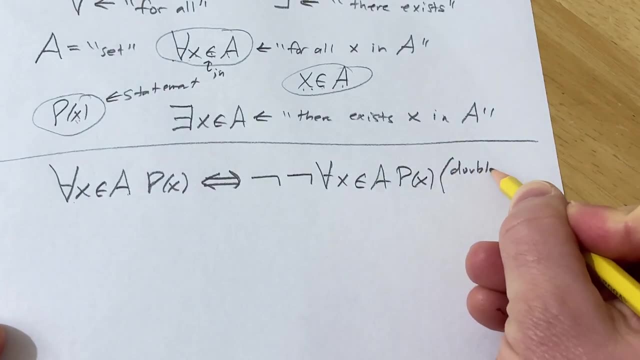 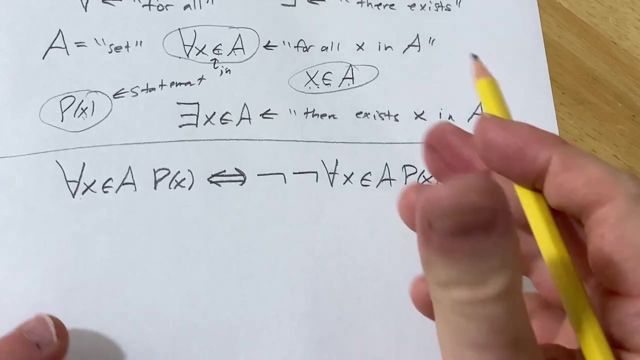 So common sense should tell you that the opposite of the opposite is what you start with, And that's exactly what this says here In mathematics, people give this a fancy name. They call it the double negation law. All of these logic laws have rules and names in mathematics, and they're all. 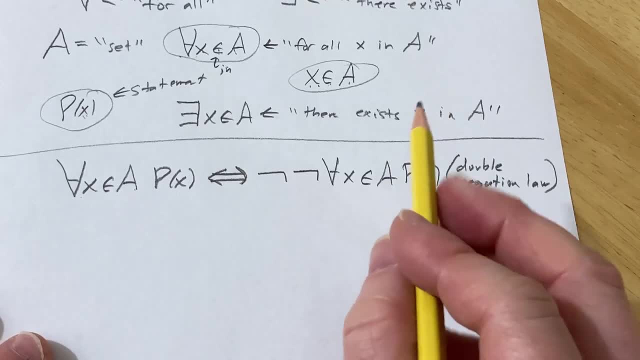 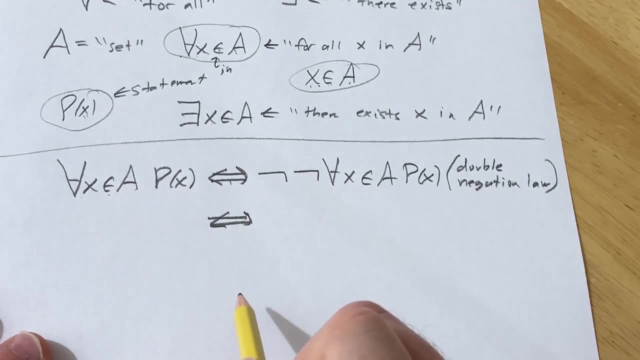 described in the book that I was talking about before. All right, so now what we're going to do. by the way, this double arrow is an equivalence arrow. It means that whatever I write here is the same as what I write here. So this is the same as, so I'm going to keep this one. 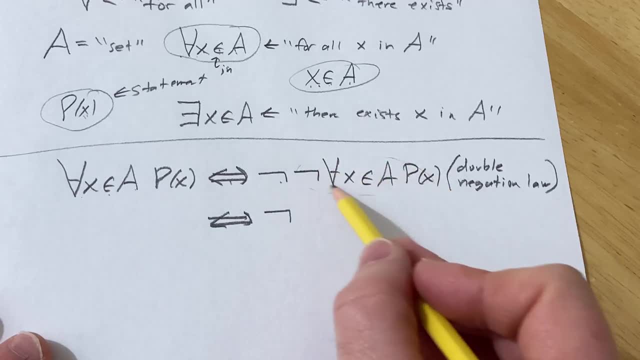 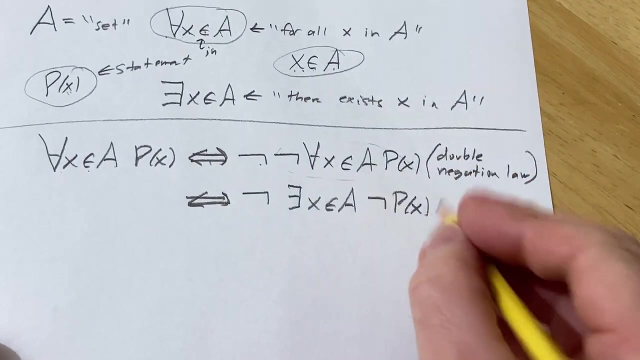 and I'm going to distribute this one through: Okay, so the opposite of this statement is there exists an x and a, such that p of x is not true. So this is something that you would need to you know, learn in a mathematical logic class to fully understand this. So, if you just believe me, 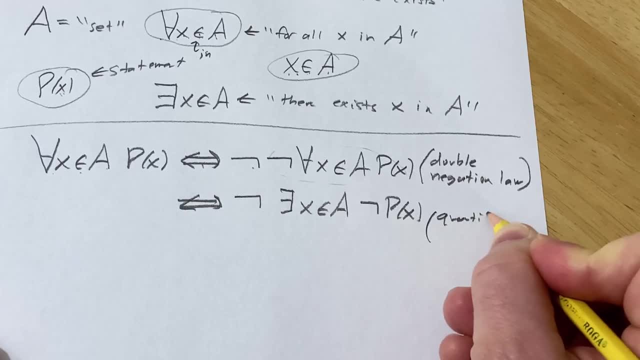 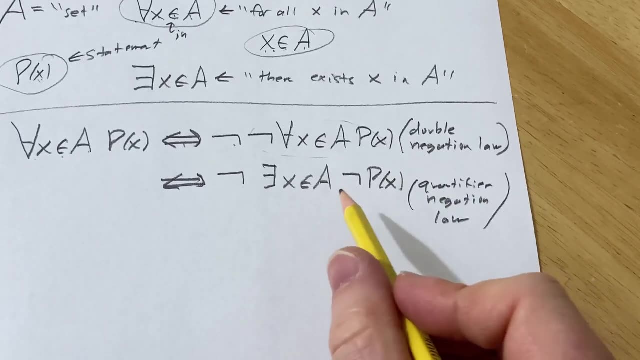 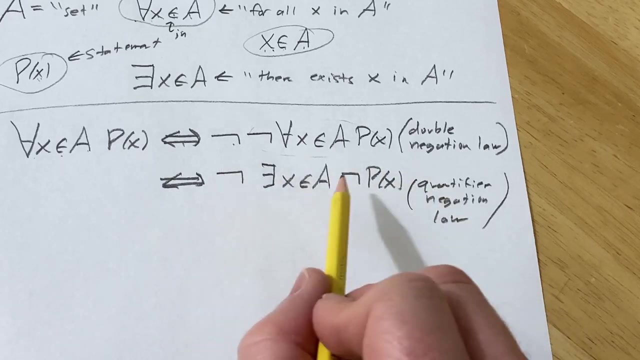 that it's true, everything is good. So quantifier negation law: This is one of the most important ones. by the way, If you ever study calculus and you do proofs in calculus, this is really, really important. Like to negate the definition of a limit. this is the one you would use, right? 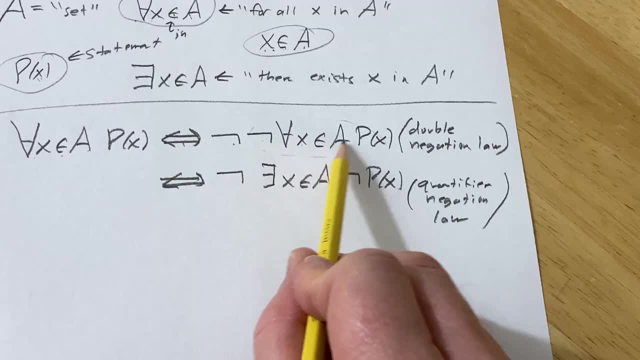 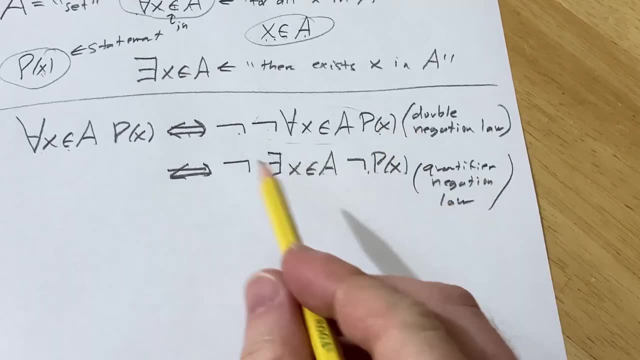 You're negating a for all statement. So for all x and a p of x. the opposite of that is, there exists an x and a, such that p of x is false. Now here's the thing: If a is equal to the empty set, 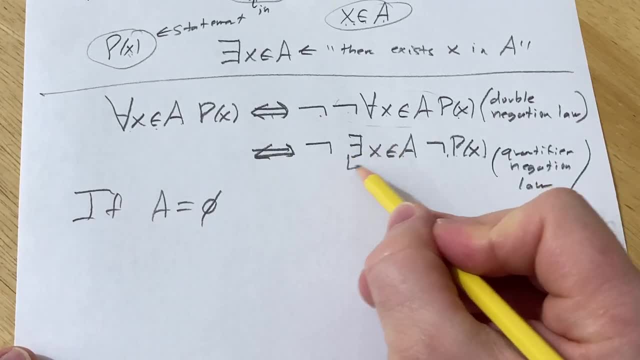 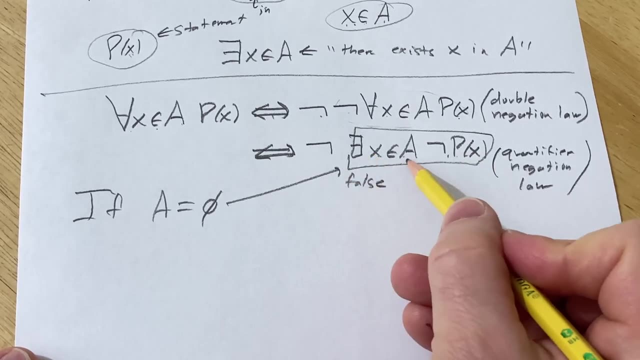 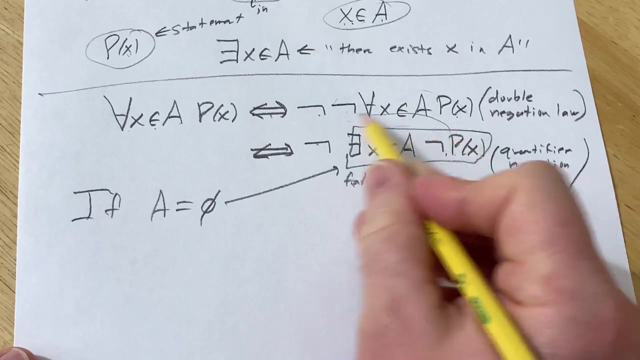 okay, so if a is actually the empty set, there's nothing in it, but this can be true. So if this is true, then this is false, right? Because there's no x's in a, so there can't exist an x and a. so this is false, But the opposite of false is true. So this whole. 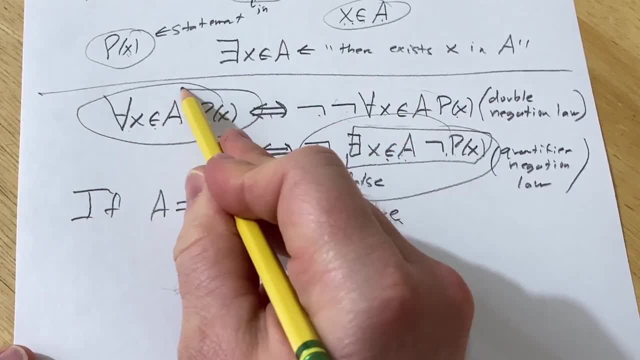 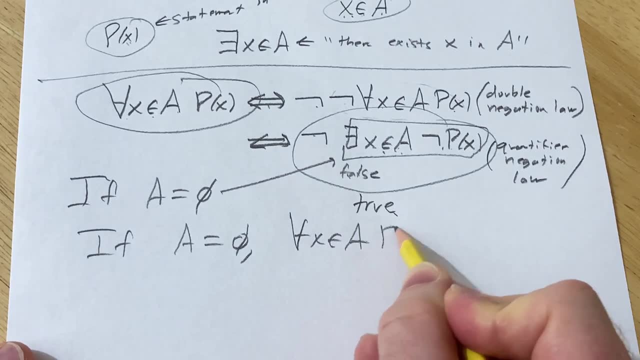 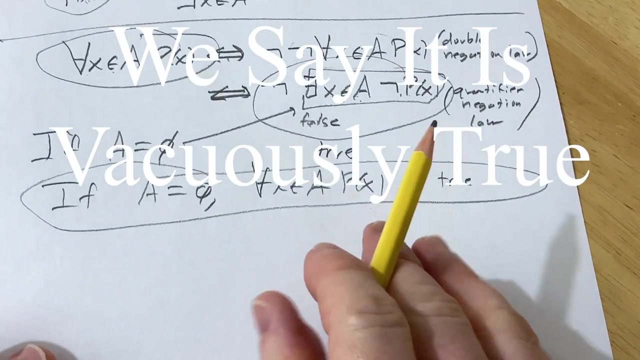 thing becomes true. That means this is true. So if a is empty, the statement for all x and a p of x is true, And that's the key, right? That's the key, That's the key behind everything in this video, And this is super key. So for 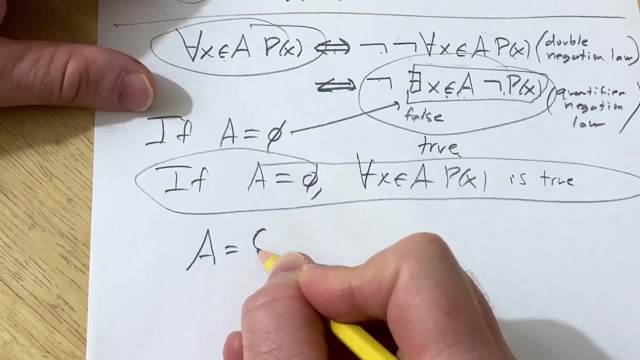 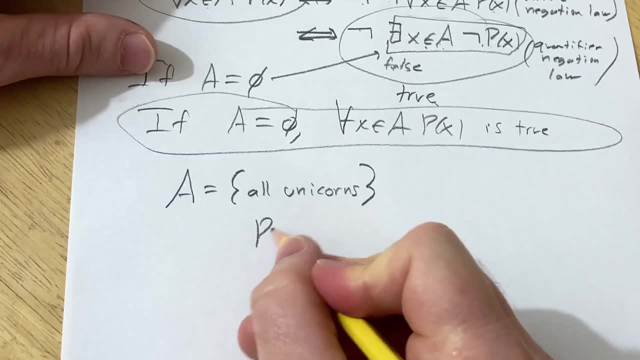 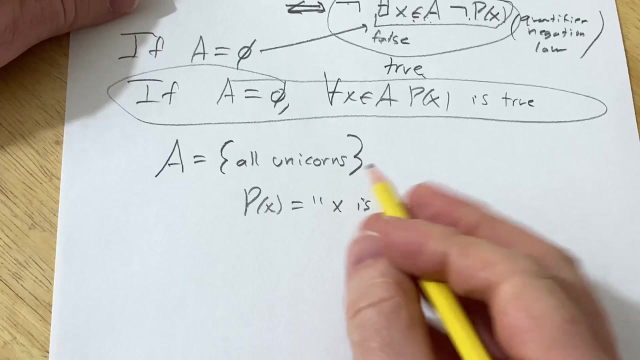 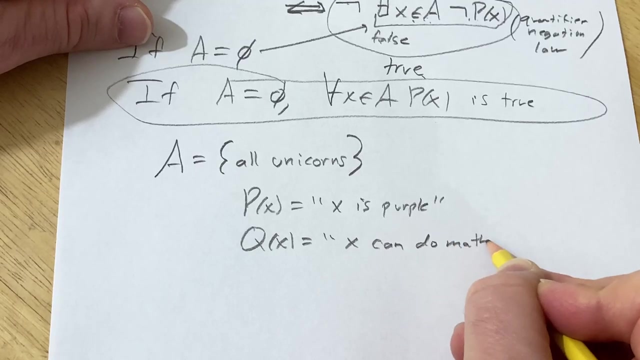 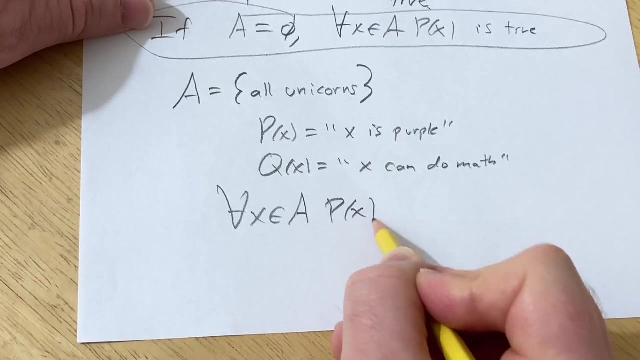 example, if I let a be the set of all unicorns and I let p of x be the statement x is purple And just for fun we'll do q of x. x can do math. Then if we look at the statement for all x and a p of x, this is saying that all unicorns are. 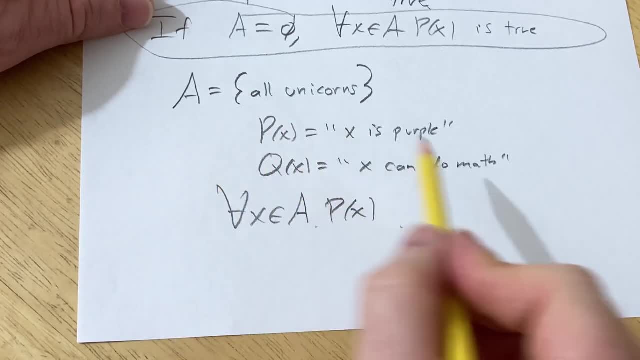 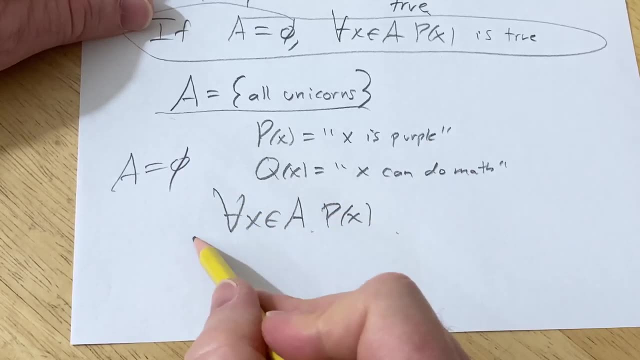 purple. But is this statement true? And why is it true? Well, it's pretty simple. There are no unicorns. Unicorns don't exist. So a is equal to the empty set. Therefore, all unicorns are purple. 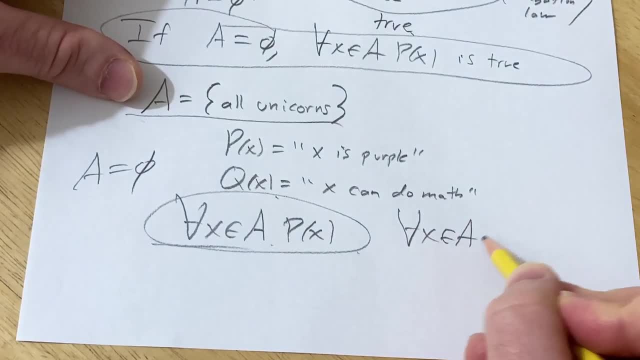 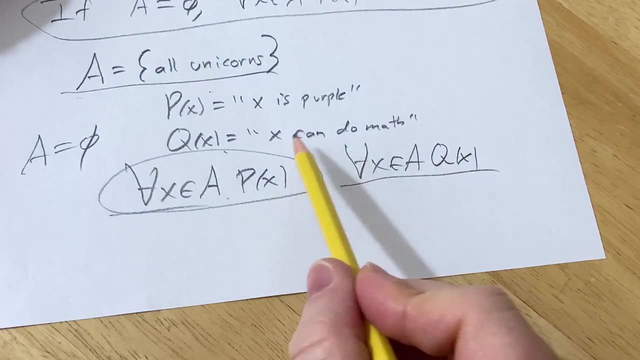 Same thing here. If I write for all x and a q of x, same thing, right? Unicorns don't exist. The empty set. So for all x and a q of x, is true. So that means that all unicorns can do math. 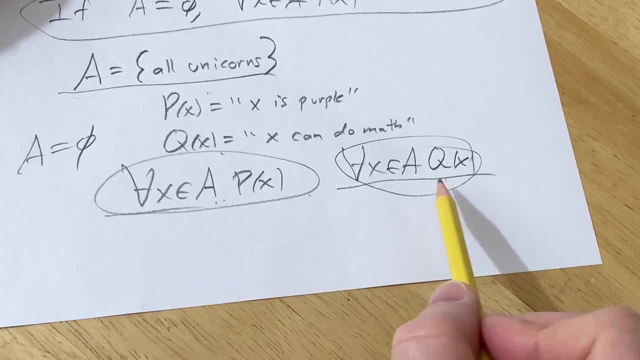 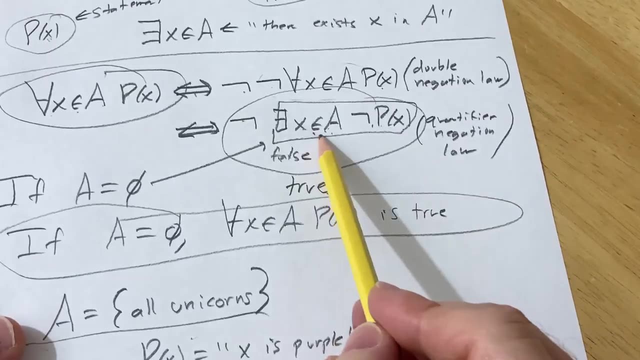 So this statement says that all unicorns are purple And this one says that all unicorns can do math, And both of these are true mathematically by what we investigated here, And this idea is explained in the book I was talking about. So it's a really awesome book.